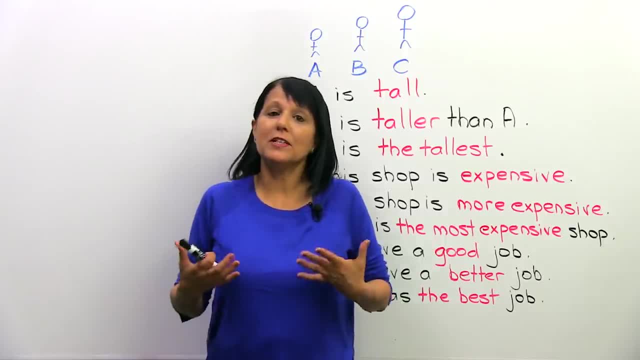 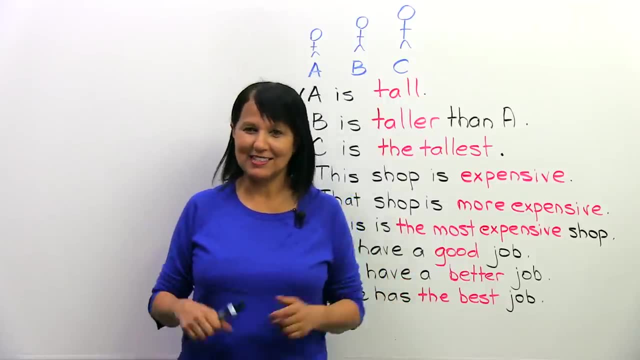 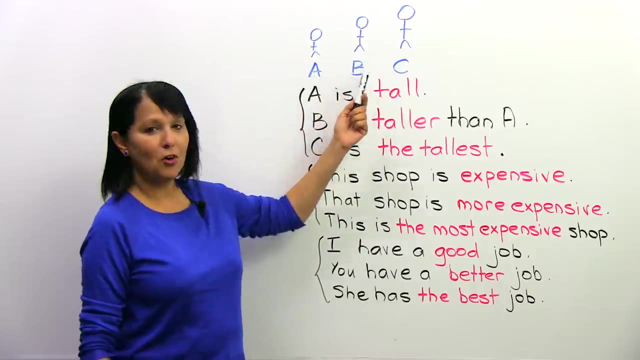 that means and how we use it. Okay, But in terms of real life, this lesson is really about something that you need to do in English almost every day, So let's get started Now. let's look at the board here, where I have tried to draw three tall men: A, B and 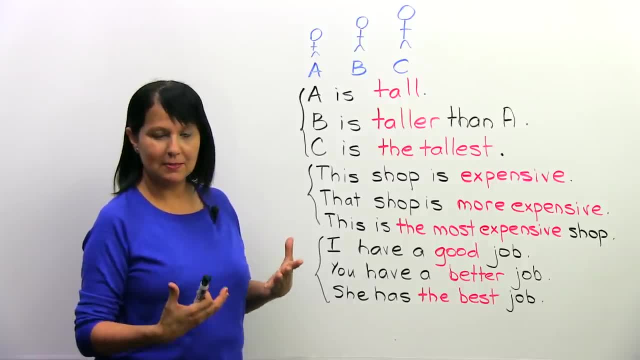 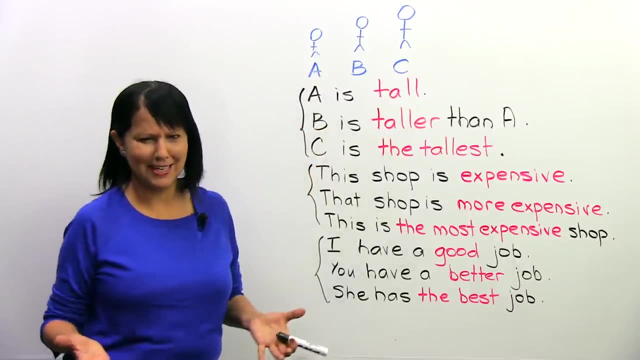 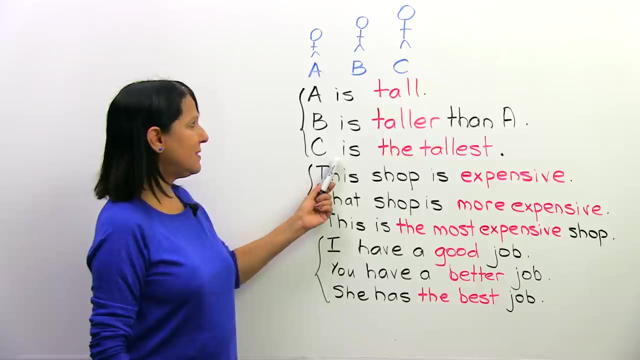 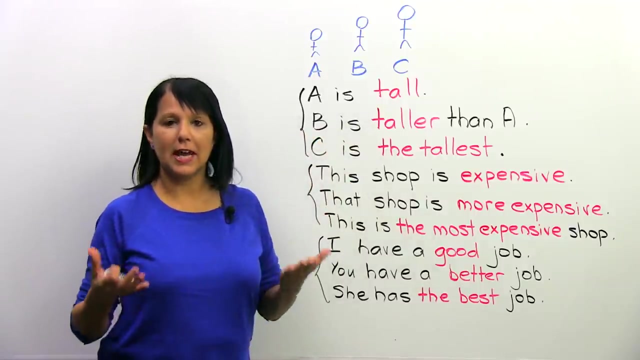 C. Now, if we describe these three people, we could say these sentences: A is tall. let's say: B is taller, C is taller than A And C is the tallest. Now, when I said A is tall, I just used an. 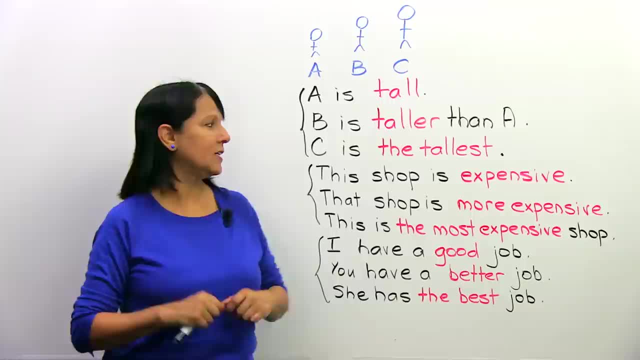 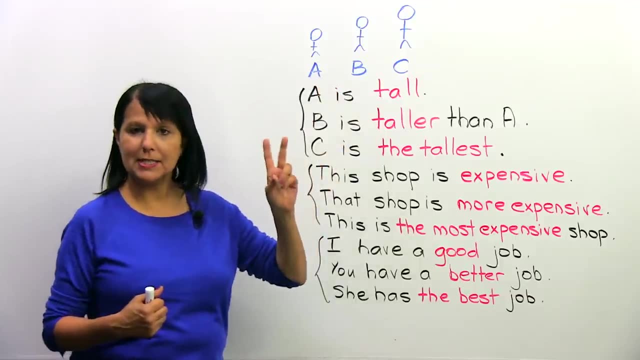 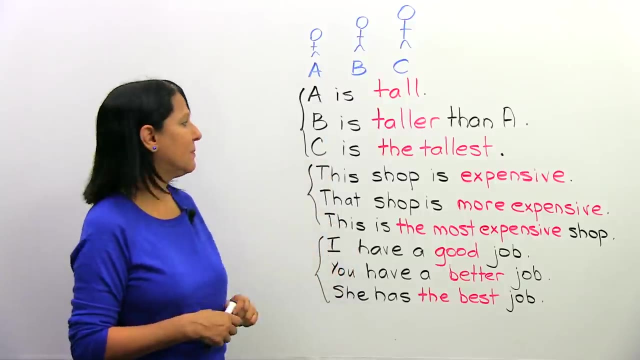 adjective tall. That's our basic adjective. When I said taller, that is when you compare two people or places or things, So that is called a comparative adjective. It compares two things. And when we said C is taller, that is when we compare two objects, So that is called. 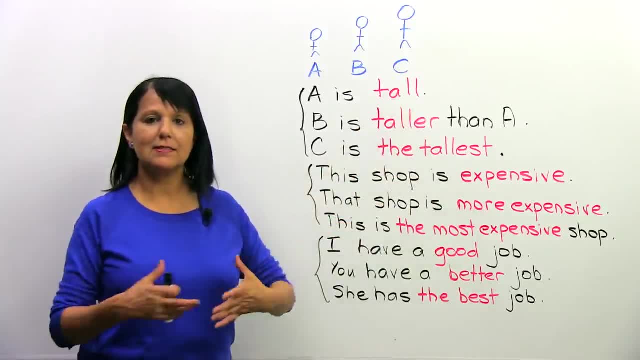 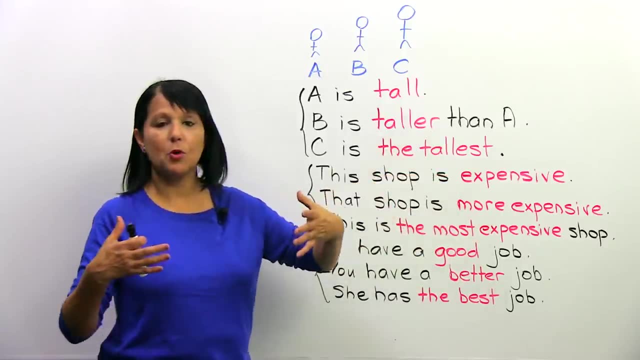 the comparative adjective. It compares two things. Now. let's say that A is taller. let's say He is the tallest. the tallest is the superlative adjective. It means the most of something. okay, In this case the most in terms of height. so it became the tallest. 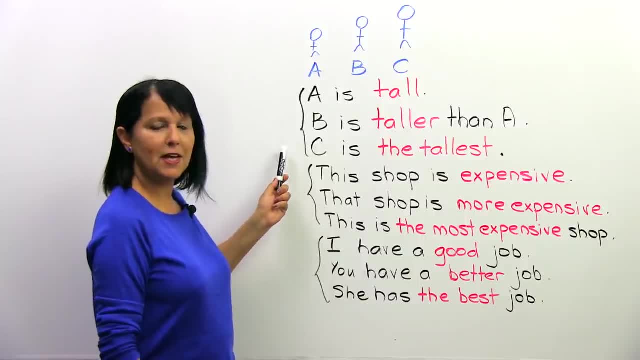 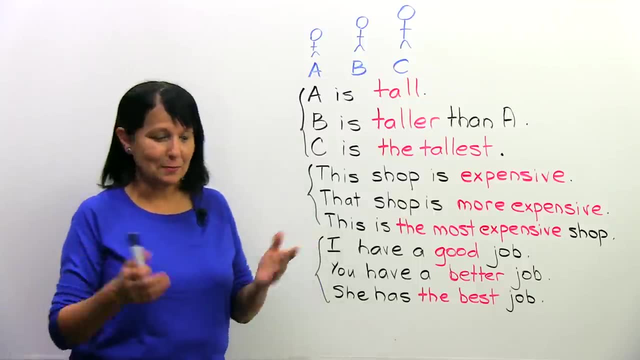 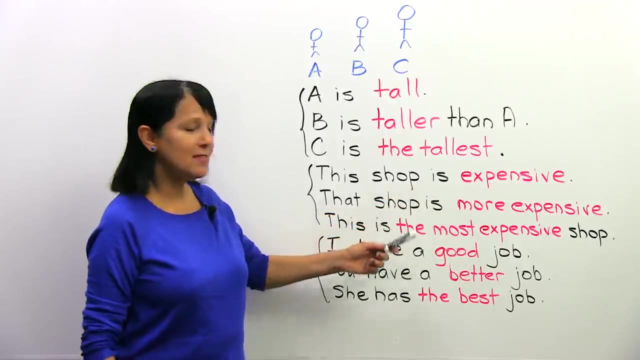 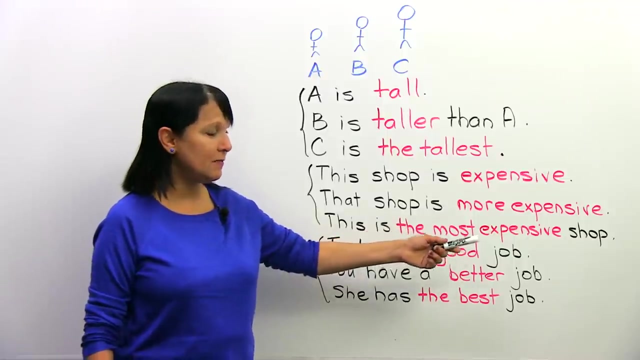 So basic adjective, comparative adjective and superlative adjective. Now, that's one way to do it, but let's look at another example. This shop is expensive. basic adjective, That shop is more expensive. the comparative adjective: And this is the most expensive shop. that's the superlative adjective right. 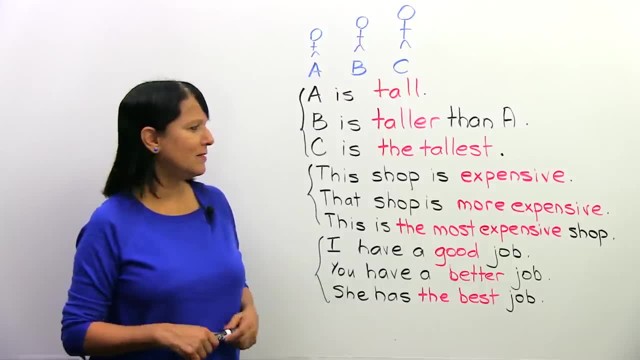 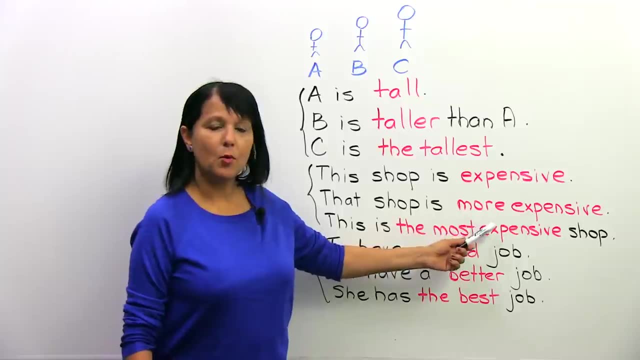 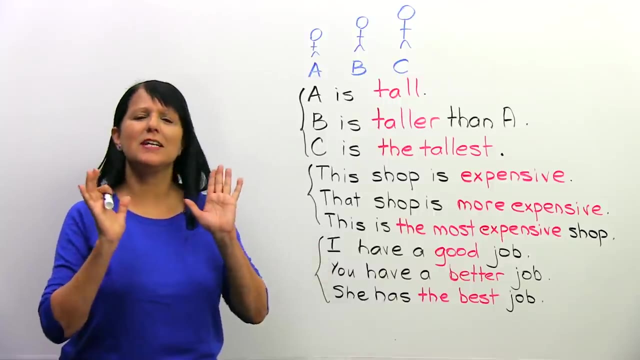 The most. But what's going on here? Here we said tall, taller, the tallest. Here we said expensive, more expensive, the most expensive, Something different, right? Okay, I'll explain to you exactly when you use this kind of construction and when you. 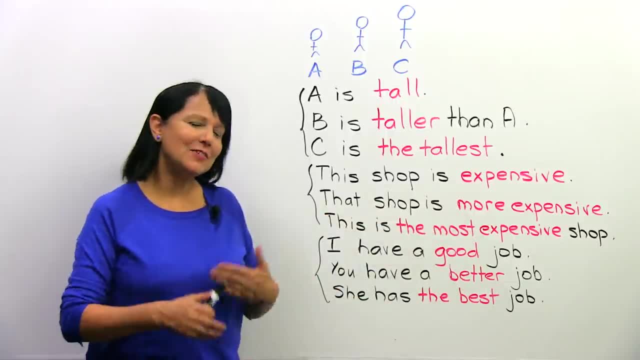 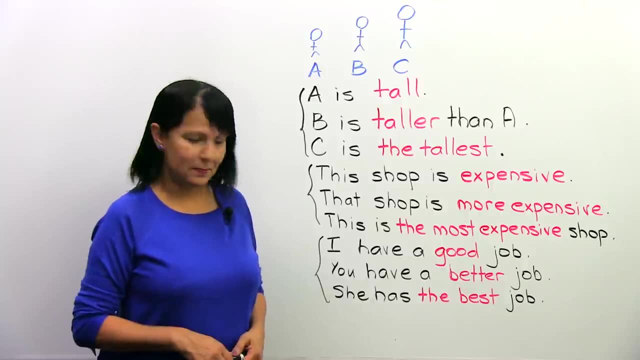 use this form. Hang in there. And let's look at one last example. I have a good job, You have a better job And she has the best job. In this case, good was the basic adjective, better is the comparative adjective. 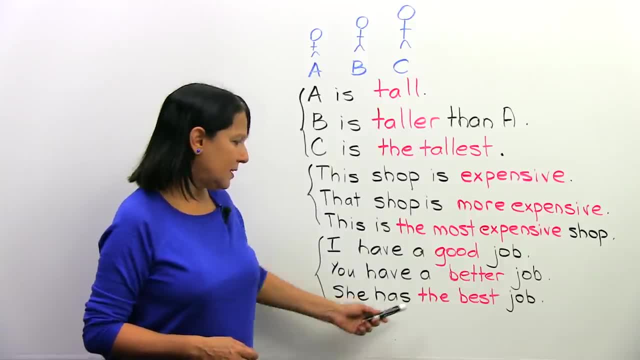 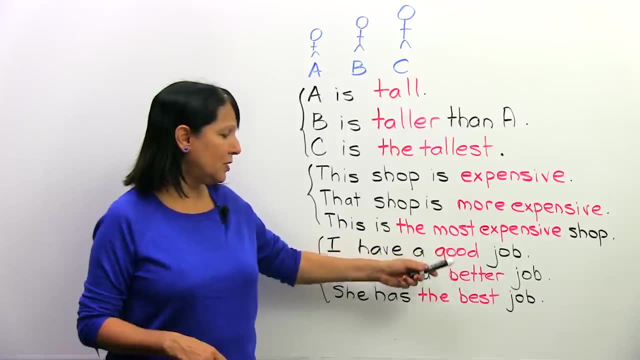 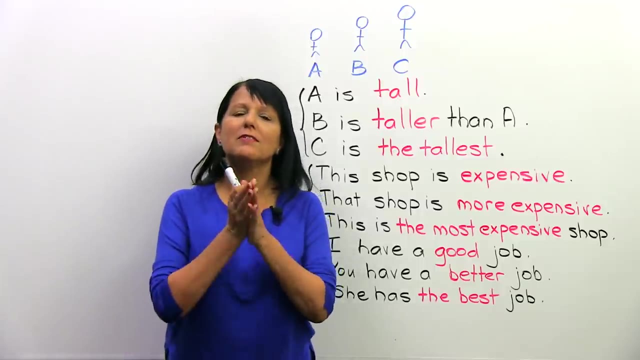 Between two people, And the best is the superlative adjective. Now we have something even more different: right, Good, better and the best. So which of these do you use when That's what you're going to learn really, really well and in such an easy way that? 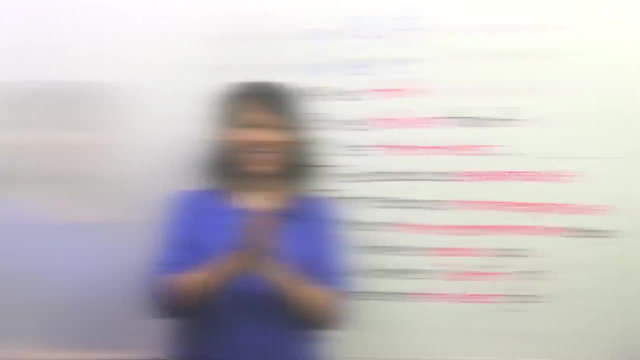 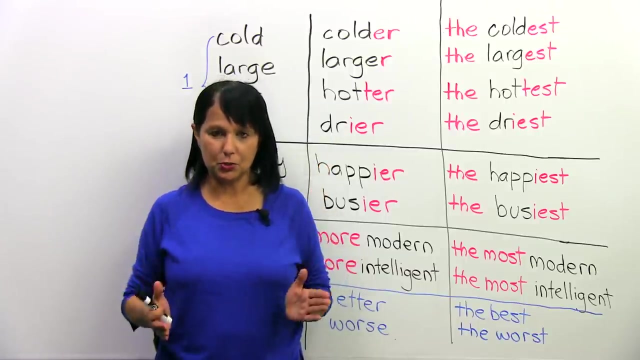 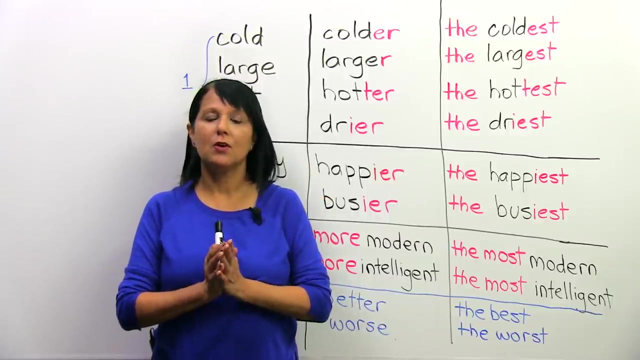 you will never forget it in just one second. Okay, so all of the examples we looked at just now were correct. So how do you decide which one to use? I'm going to show you now with a very simple chart, And what this chart shows you is that the point that matters is the adjective itself. 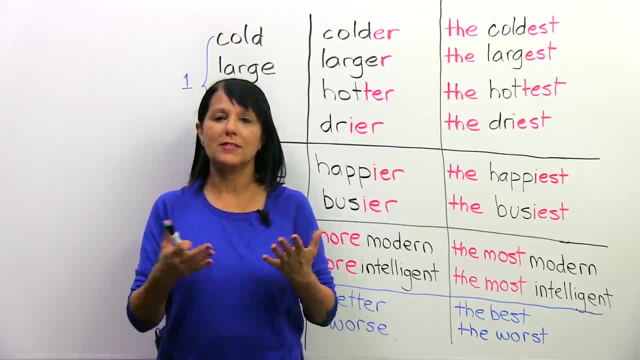 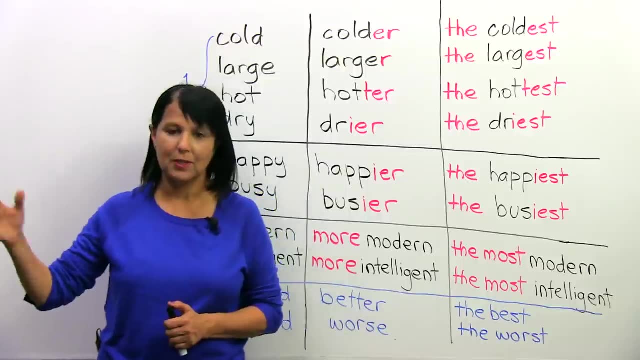 how many syllables is it divided into? What's the syllable It's? how many parts, in terms of pronunciation, is the word divided into? And I will explain that to you right now. So When we look at a very short word, 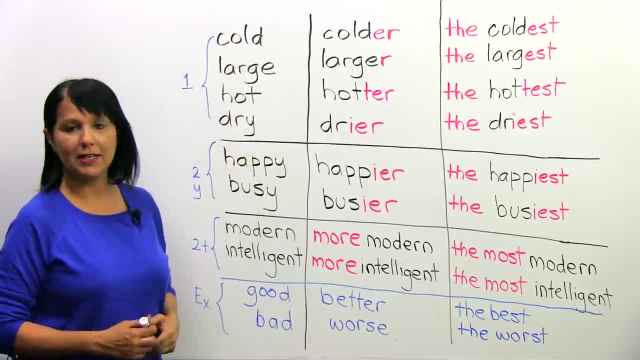 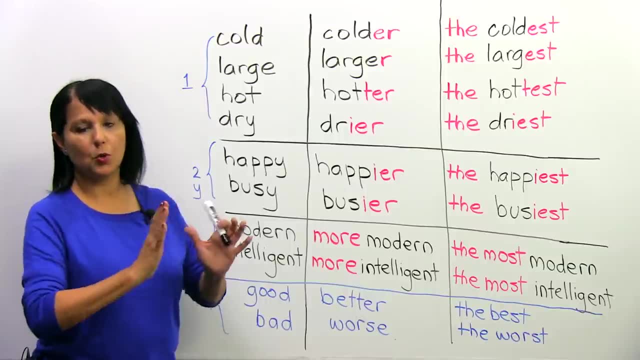 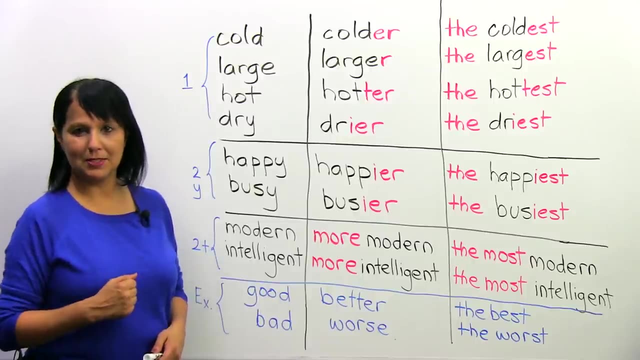 Like cold, large, hot or dry, it has only one syllable. We say it fast cold, we cannot say cold, we just say cold. So it has one syllable. When we say this word happy, it has two syllables. 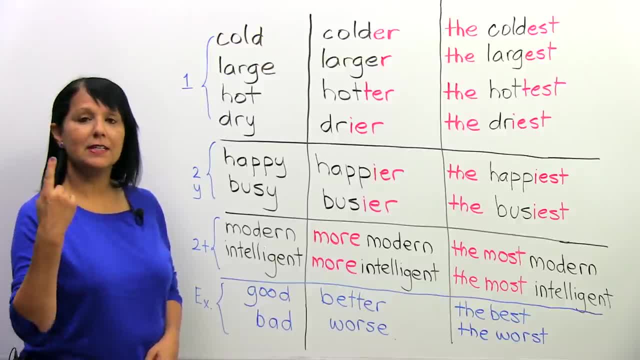 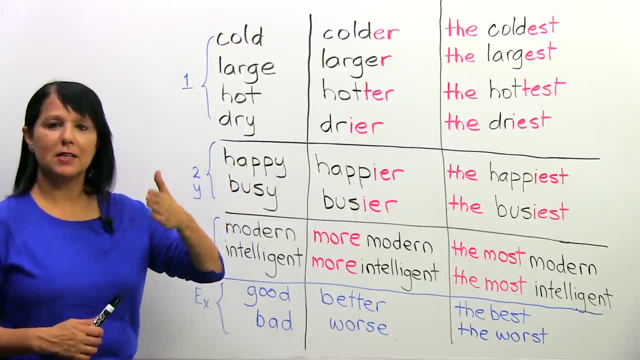 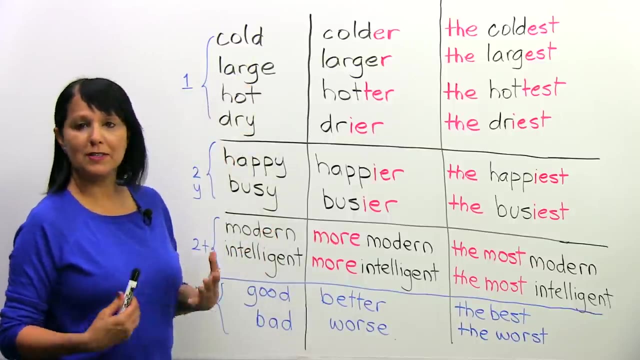 When we say this word intelligent, it has intelligent- four syllables actually. Okay, So syllables are just how many parts Divided in two when we can pronounce it Now. so when we start with one syllable words or really short words, all you have to do 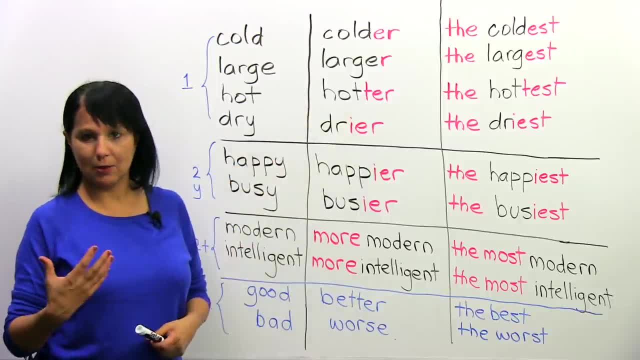 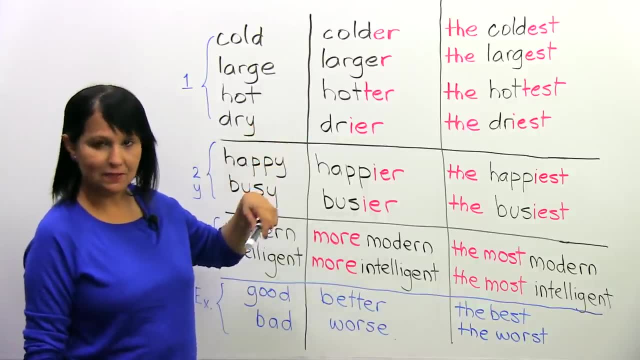 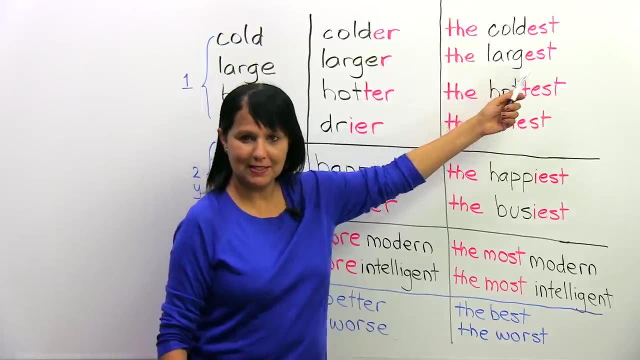 is to add an ER sound. So, for example, the basic adjective is cold, the comparative adjective is colder and the superlative adjective is the coldest. Cold, cold, Cold, cold. Okay, Colder, the coldest. 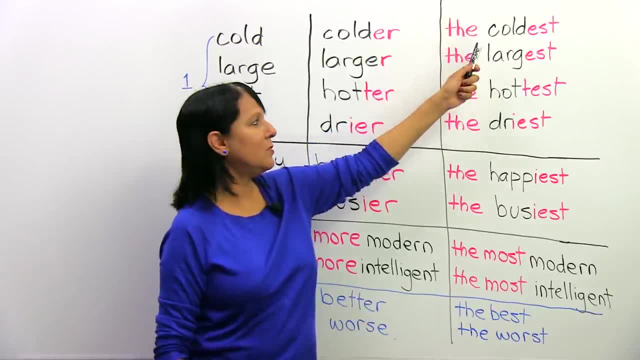 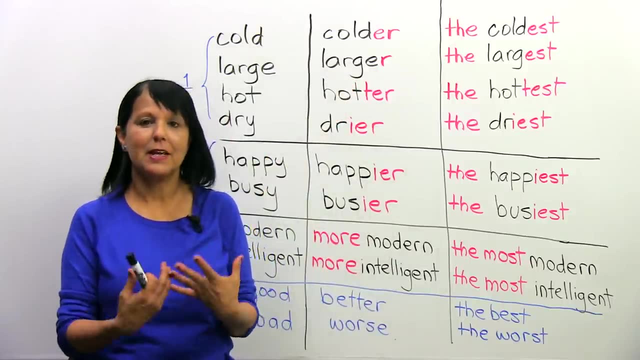 Now remember, when you say this one, don't just say coldest, remember to say the coldest. Whatever I've written on the board in red is what you need to add. Now there are two different things: One is when you're speaking and one is when you're writing. 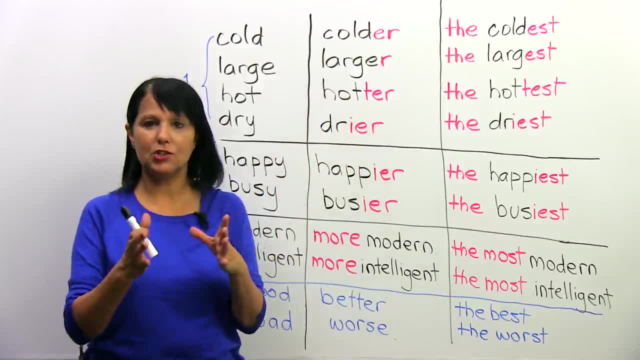 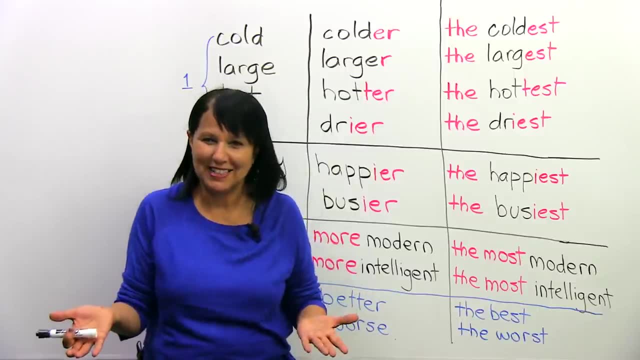 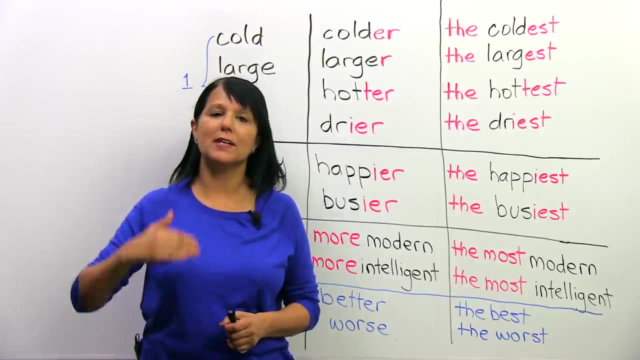 So you will see here on the board that there are some changes you need to make in spelling. But first of all learn what to say, because in the saying of it you don't need to spell anything. All right, Later you can download a free resource that I've written that will explain to you exactly. 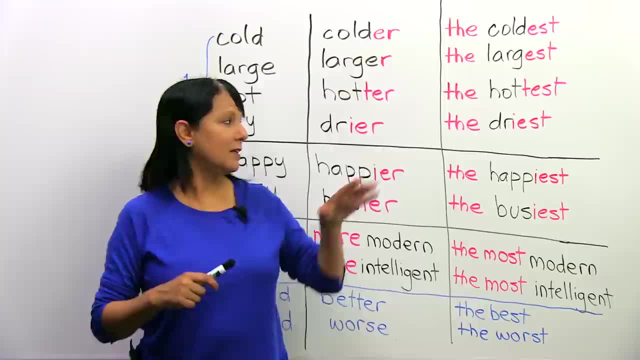 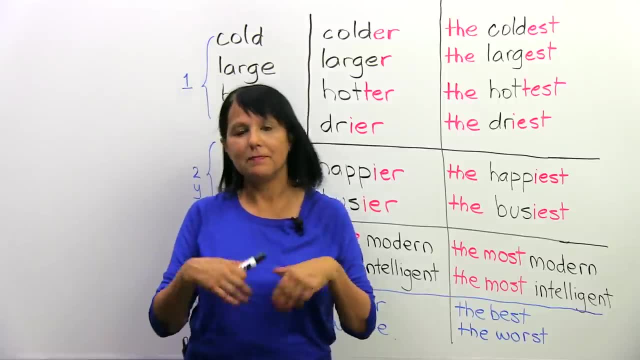 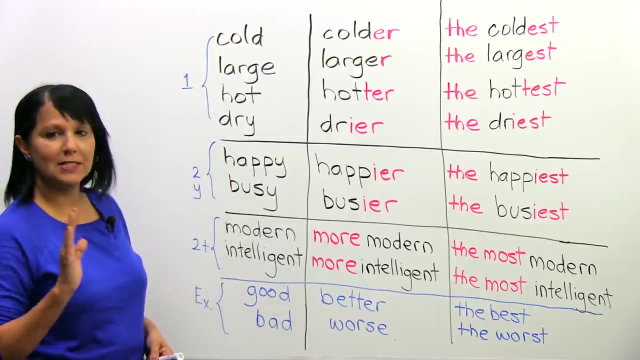 all of the changes you need to make, also in the comparison and also in the spelling. All right, But that's later. Now let's just look at and understand the basic principles. So one syllable short words are just like that. 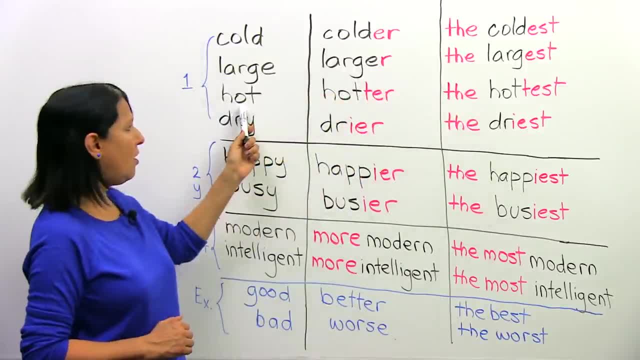 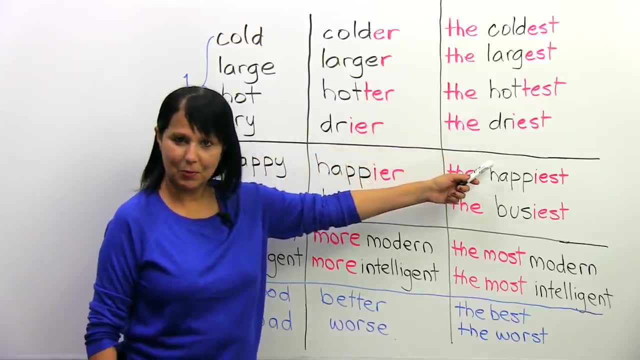 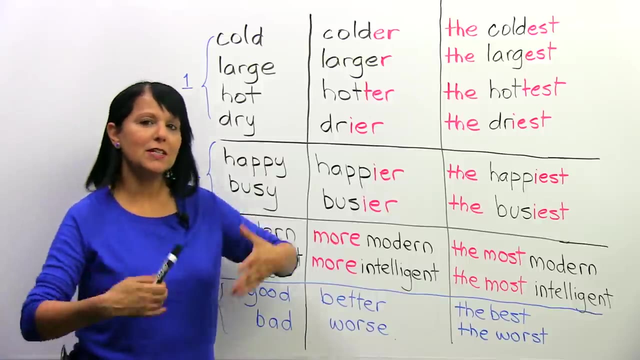 Large, larger, the largest- Okay, Hot, hotter the hottest. Dry, drier- the driest- Okay, Yes, there are spelling changes, but again refer to the reference sheet for that. Right now, just try to get the rhythm of it. 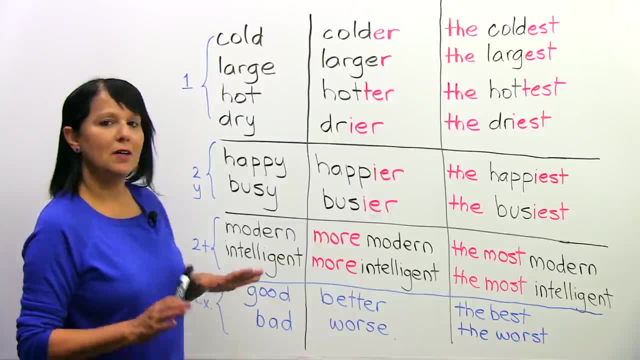 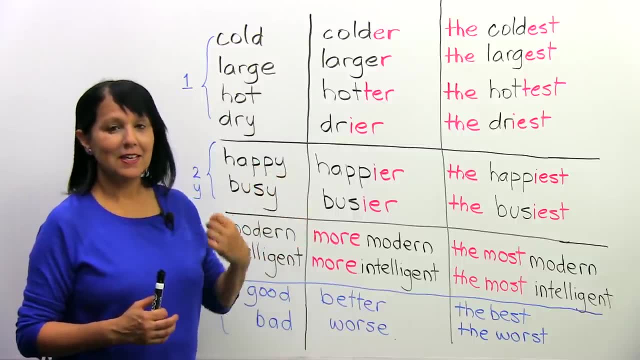 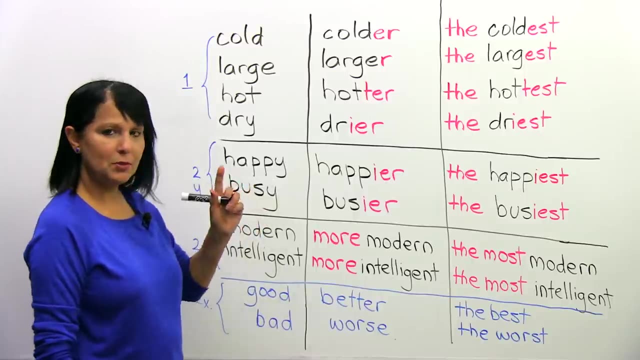 Okay, Say it out loud with me Now. the next rule is: when you have a two-syllable word which ends with Y, then we do this. So let's take this example: happy two syllables, happy ending with Y. so we cancel the Y and 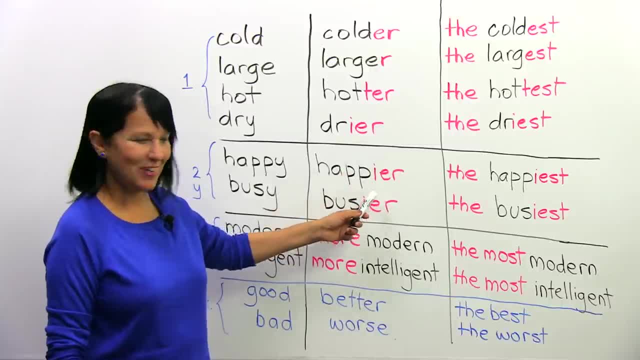 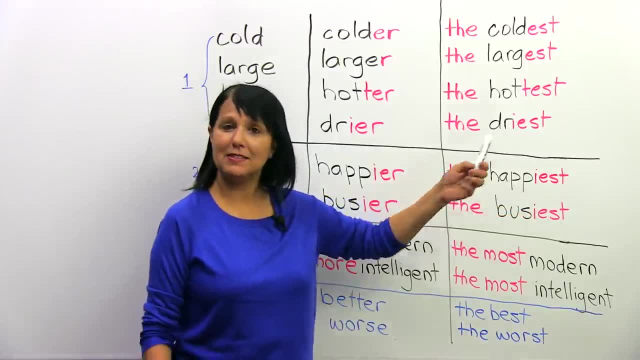 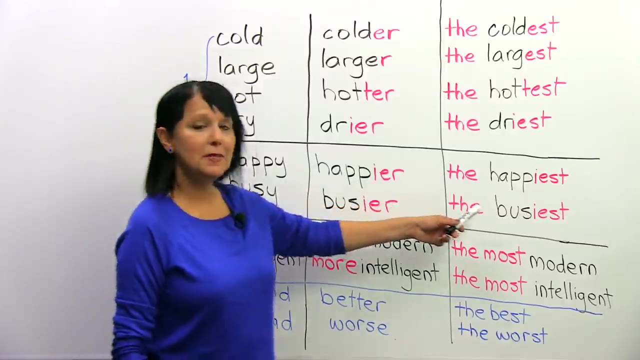 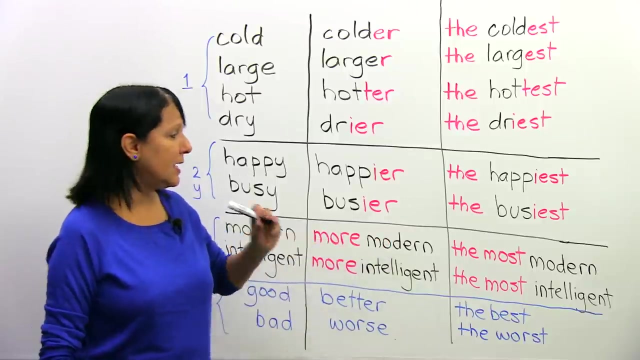 we add I-E-R. happier. Okay, Happy, happier, the happiest. This is the happiest day of my life. Okay, All right, Busy, busier, the busiest. This week I'm busy. Last week I was busier. 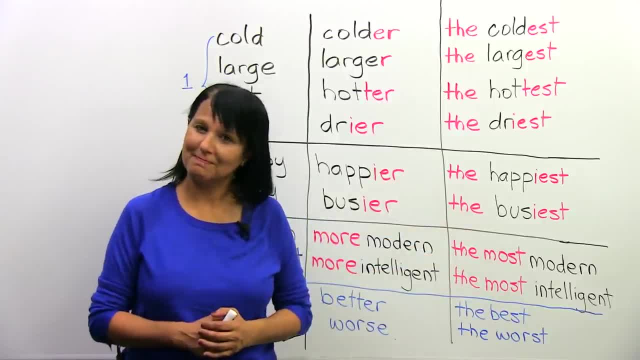 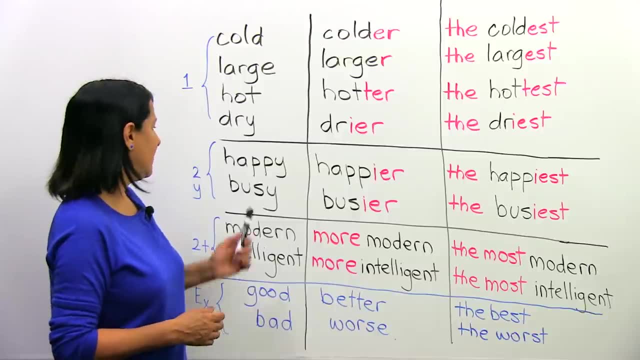 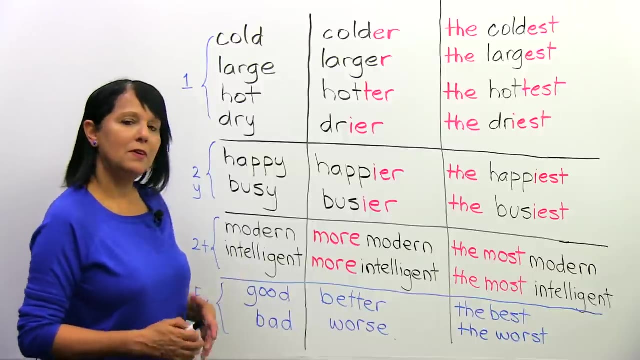 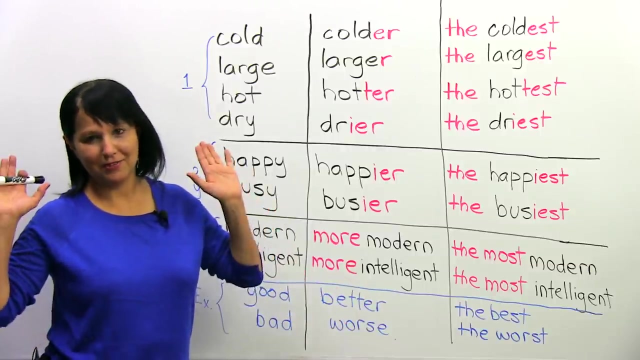 Next week will be the busiest week of the month. Okay, Like that. So one syllable, just basically E-R or R. Two syllables ending with Y, I-E-R, usually, And now for every other word which is two syllables or more, you have a different pattern. 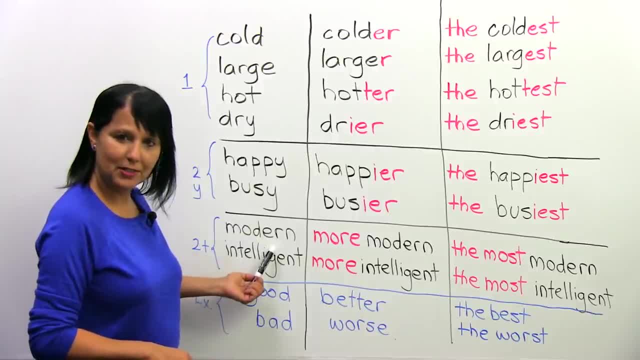 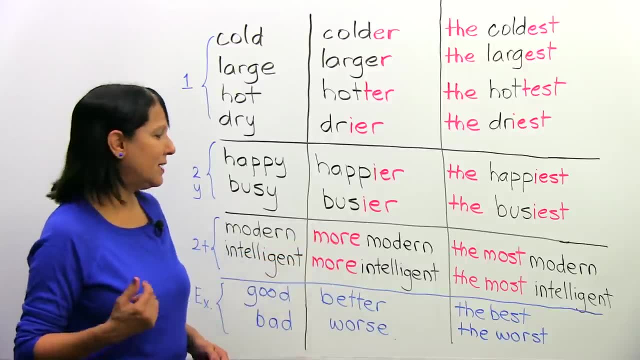 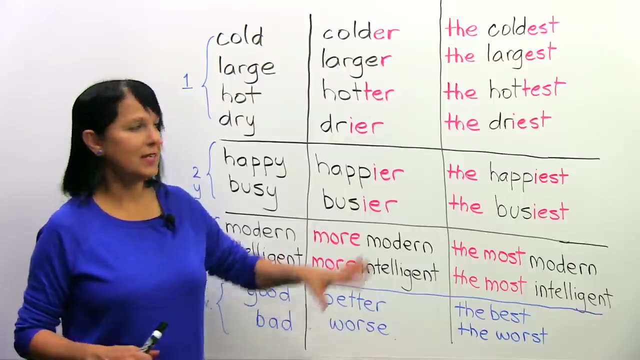 Okay. So let's take an example: modern, mo-dern, two syllables right, Modern, more modern and the most modern. Okay, So now you see where this construction comes in. right, It's different from these. 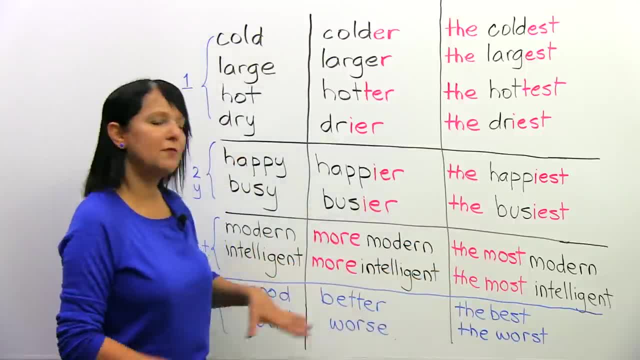 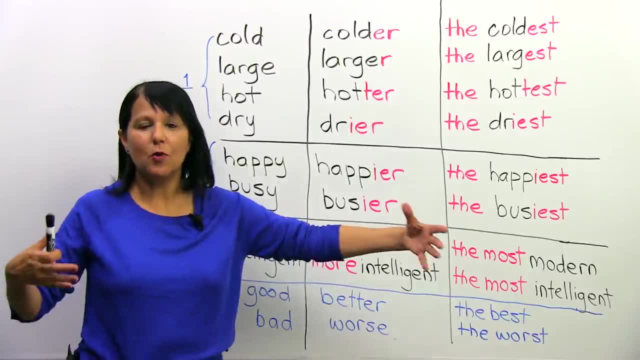 Here we're using more and the most The same for any word in English, which is a little bit long. When we say two syllables, it means two, three, four syllables- Definitely longer words. we're going to use this construction. 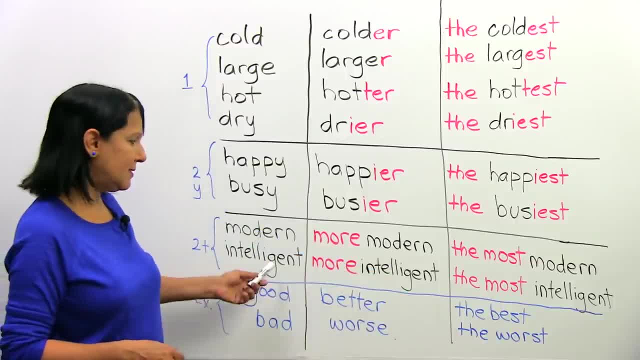 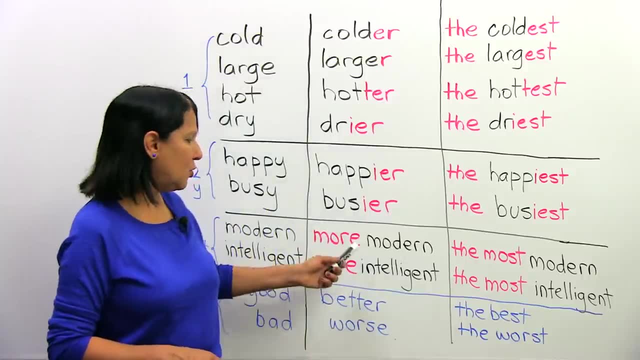 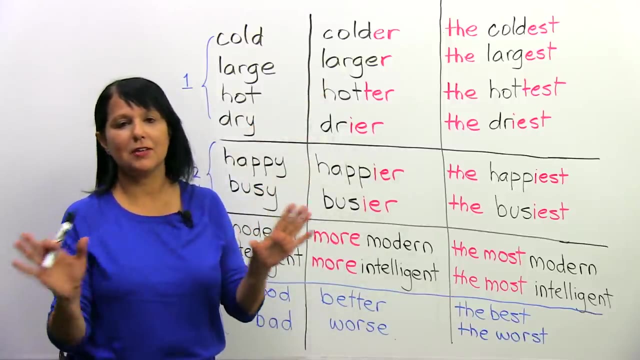 Okay, For example, intelligent, he's intelligent, he's more intelligent, he's the most intelligent. Okay, So more and the most, but we don't change the adjective itself. So those are the three basic things that you have to remember. 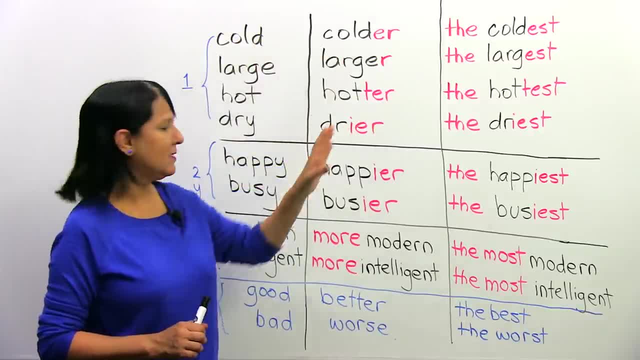 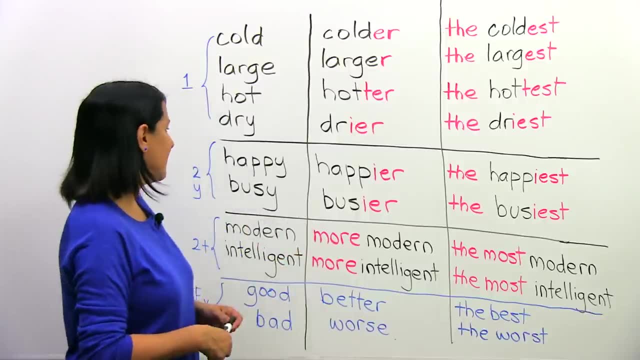 If it's a very short word, just go hot, hotter, hottest, The hottest, Hot, hotter, the hottest. Okay, When you're saying the sentence, it will come to you much more naturally: Happy, happier the happiest. 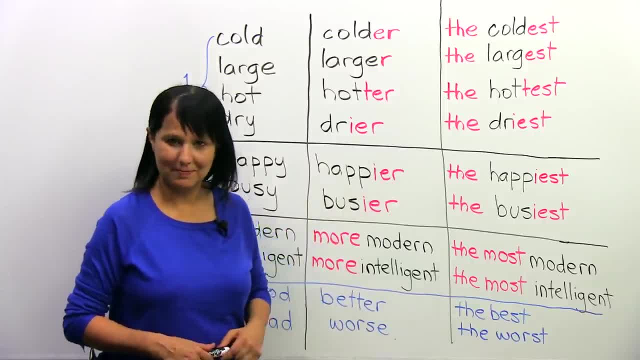 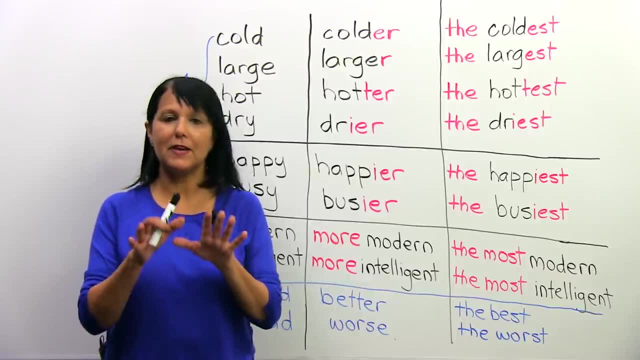 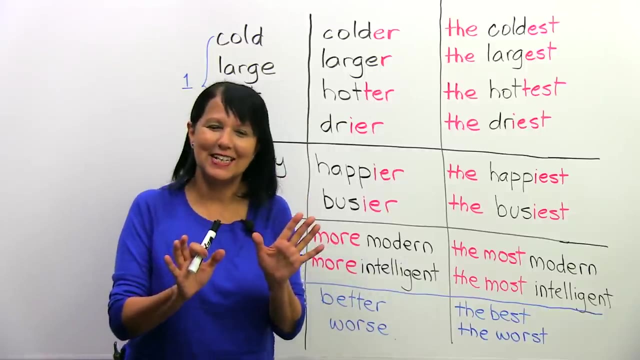 Okay, And modern, more modern, the most modern, All right, That's the rule. Those are the basic rules and that will help you with any comparative or superlative adjectives that you want to use. except for a few, really, there are not that many, a few exceptions. 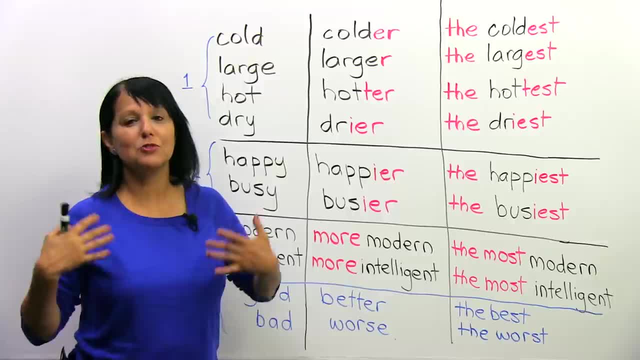 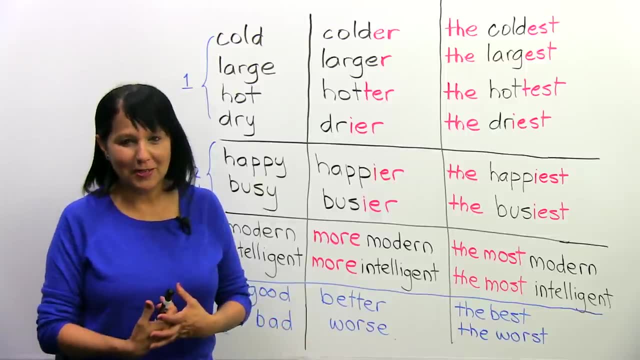 And down here I've written two of the most, So the most popular and the most common exceptions. all right, There are not too many exceptions, so don't worry, but these two are very common and you really must know them very well, because if you make a mistake with these, it doesn't. 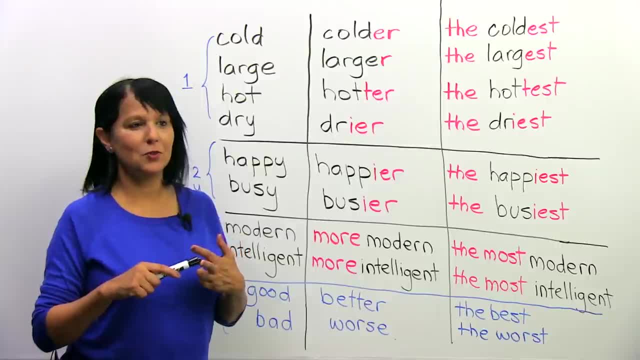 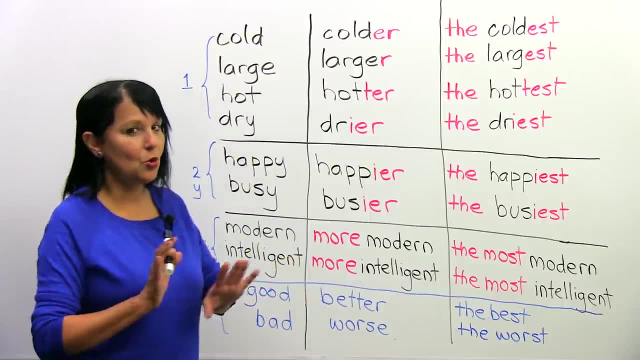 look good. Doesn't look good if you're doing an exam. doesn't look good if you're going for a job interview, or if you've written your resume or a cover letter, anything like that, Okay. So don't make any of these mistakes down here at all. 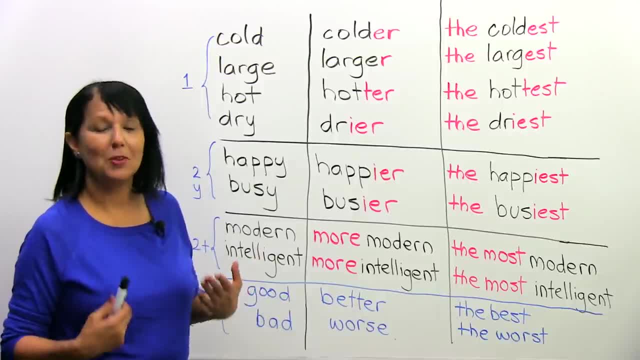 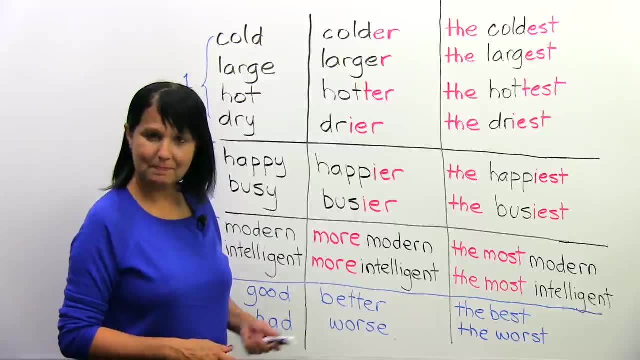 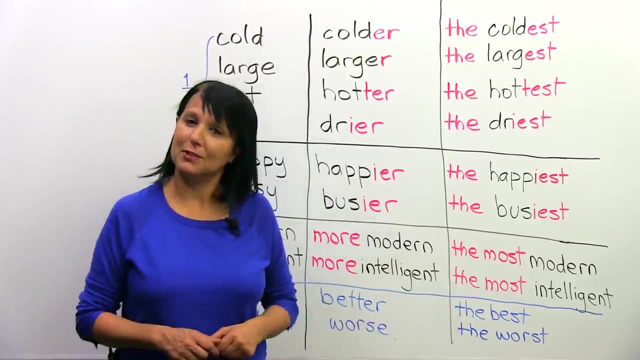 So what are these? These two very popular adjectives which are exceptions: good and bad. So the party was good, last week's party was better and this is the best party I've ever been to. So here we have good, better and the best. 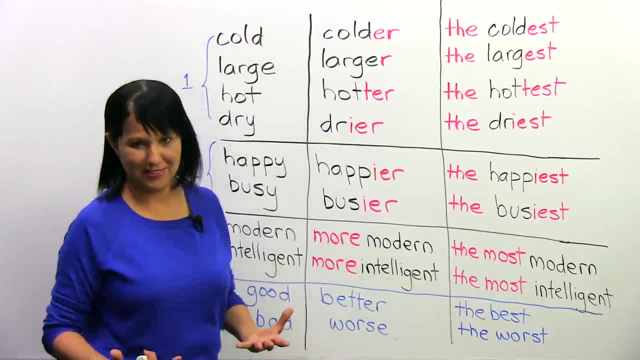 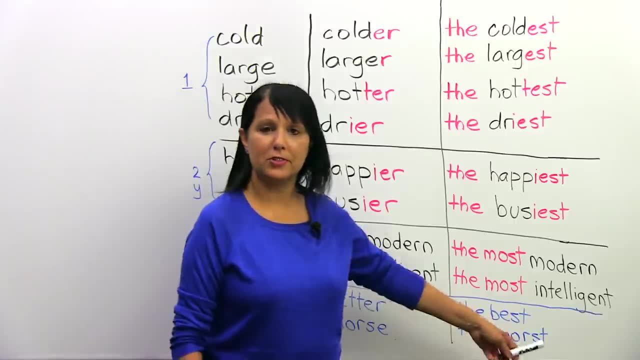 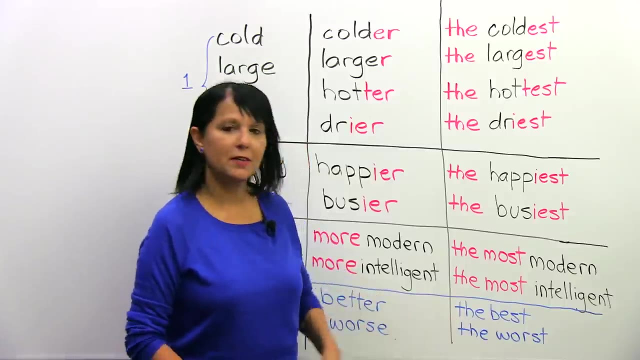 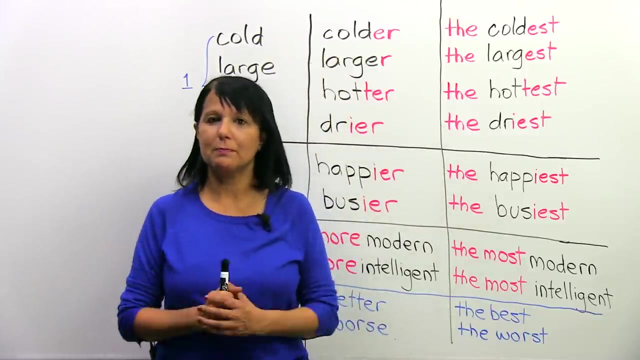 So the words actually change. We use different words. Okay, Also bad, worse And the worst. Okay, Bad, worse and the worst, And remember to use that word: the All right. So these are the basic rules. these are two exceptions. there are maybe six or eight more. 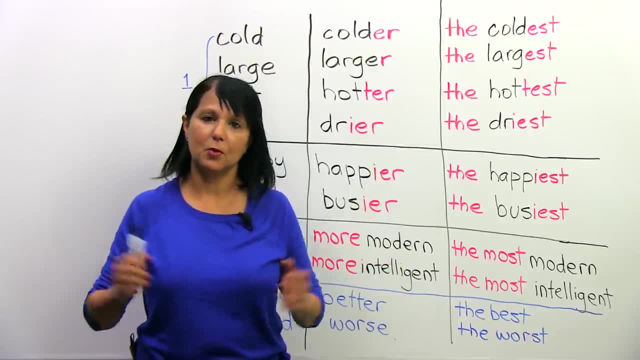 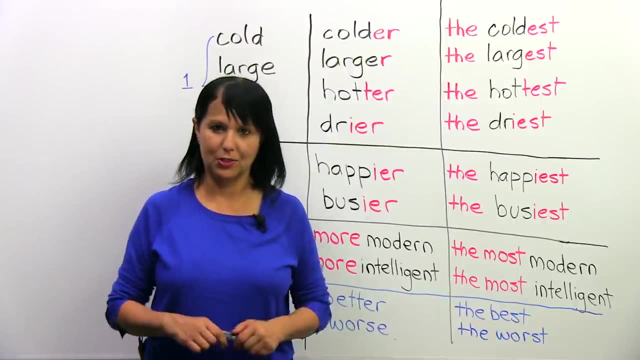 Again, in the resource which you can download for free from our website, I will have written for you most of them, almost all of them, that really matter and which you need to know, And also you'll be able to learn these spelling changes. 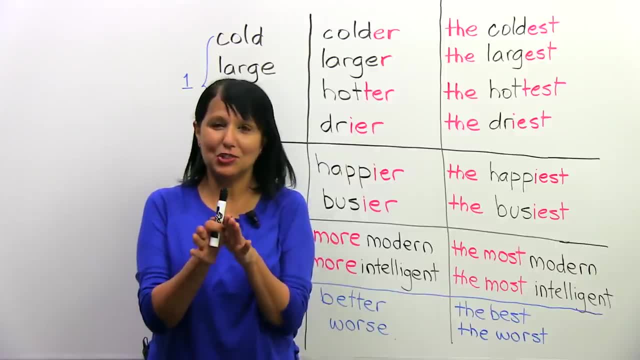 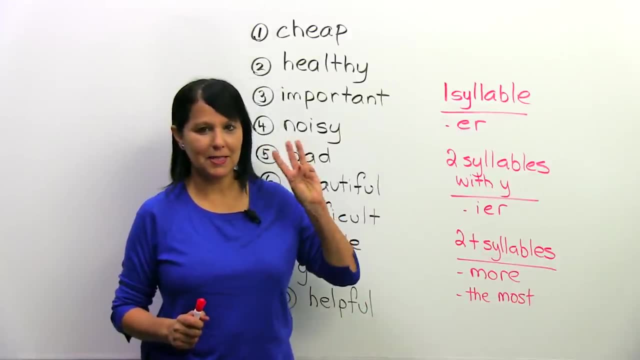 But before you go away, let's check how much you've understood by doing a short quiz. Okay, Let's do that. So as we do the quiz, remember the three basic rules. If it's one syllable. if the adjective is one syllable and short, give it a sound of. 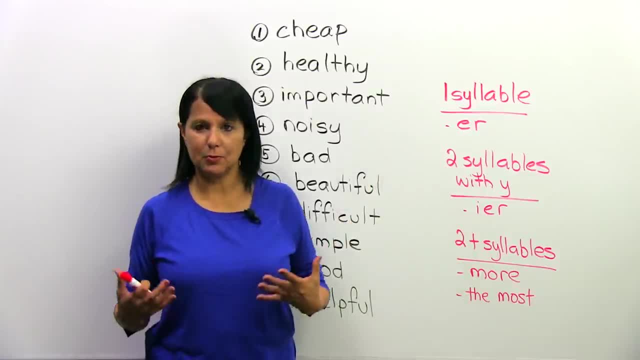 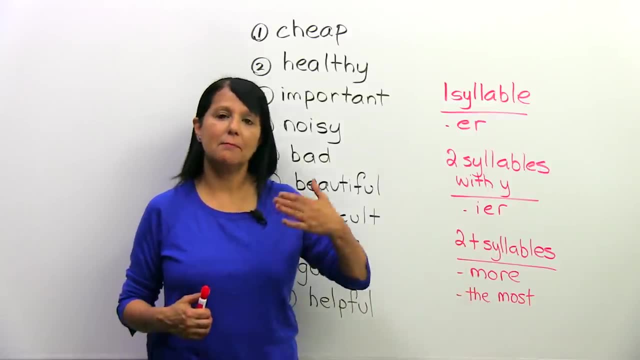 ER. If it's two syllables but ends with Y, give it an IER, And if it's two or more syllables, then we say more something, Or If it's superlative, the most something, All right. 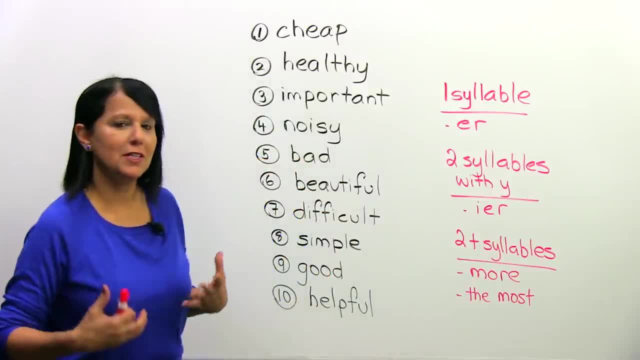 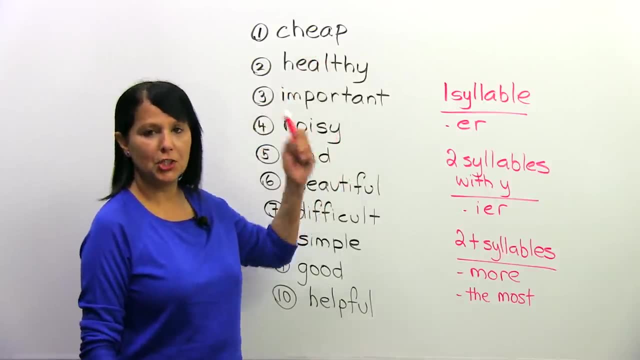 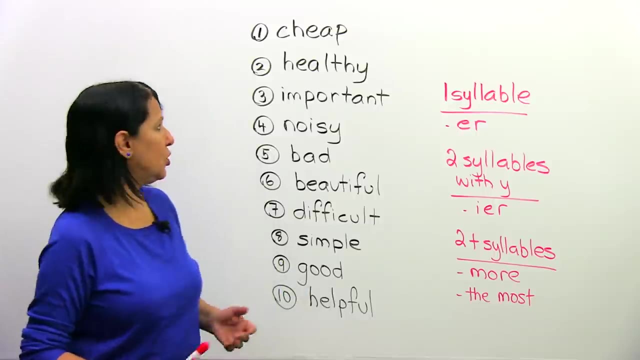 I think you've got it. Let's get the rhythm of it now by doing some examples. Here we go. The first word: cheap. make it comparative cheaper, make it superlative. the cheapest, Cheap, cheaper, the cheapest. 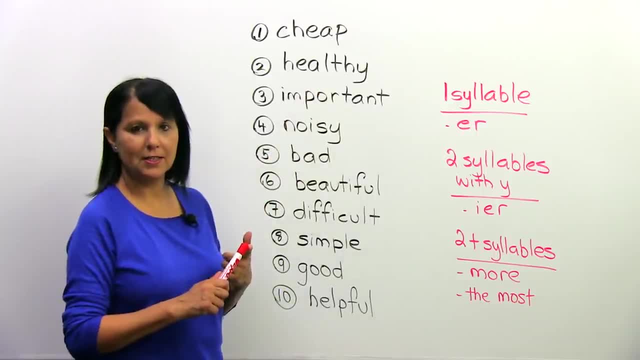 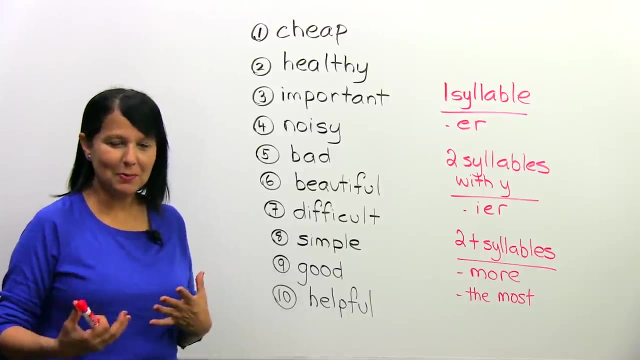 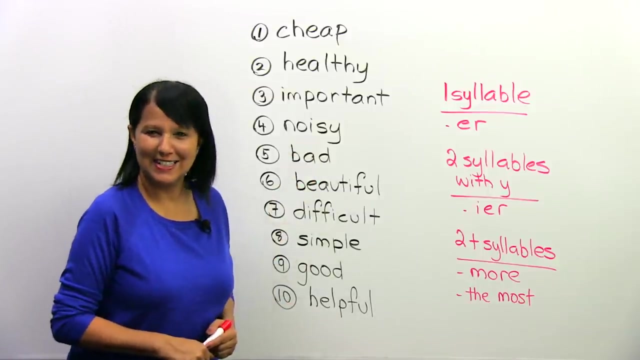 Good, Healthy, healthy, healthier, the healthiest Good, Important, Important, more important, the most important Good. Say it along with me. Okay, You might even say it before me, because you know it now. Okay, Noisy. 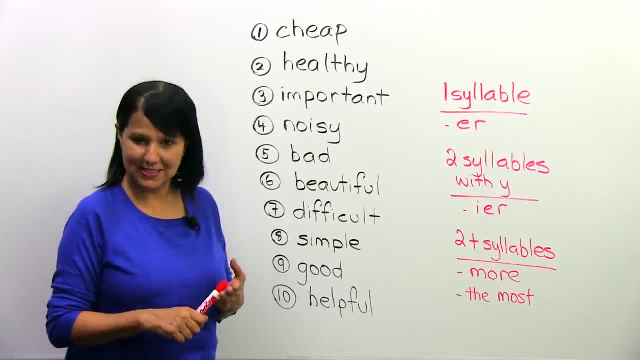 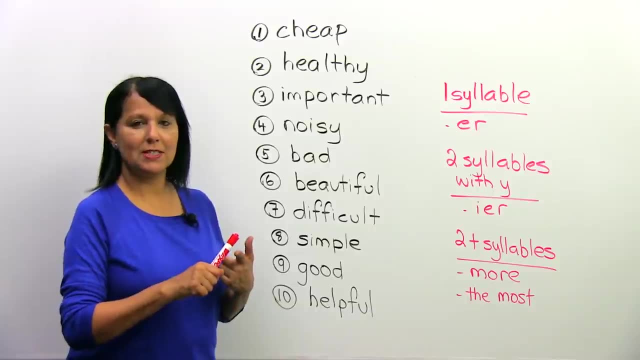 Noisy, noisier, the noisiest Bad, Remember that one. That's an exception. So we say bad, worse, worse, Bad, Bad, The worst, The worst, Good, Beautiful, Beautiful, more beautiful, the most beautiful.